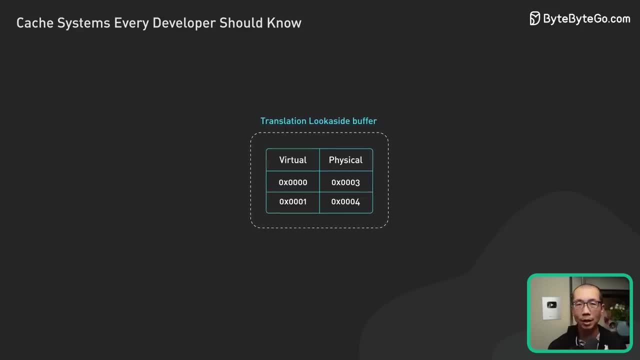 the Translation Look-Aside Buffer, or TLB. It stores recently used virtual to physical address translations. It is used by the CPU to quickly translate virtual memory addresses to physical memory addresses, reducing the time needed to access data from memory. At the operating system level, there are page cache and 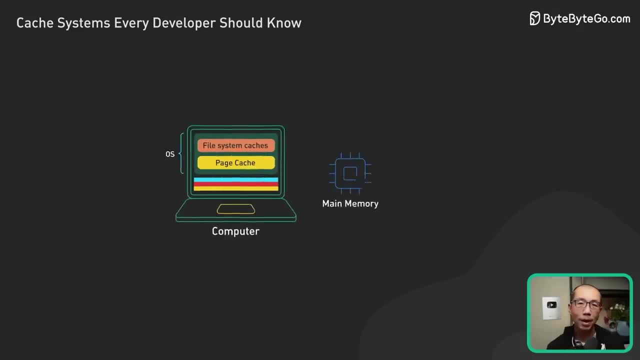 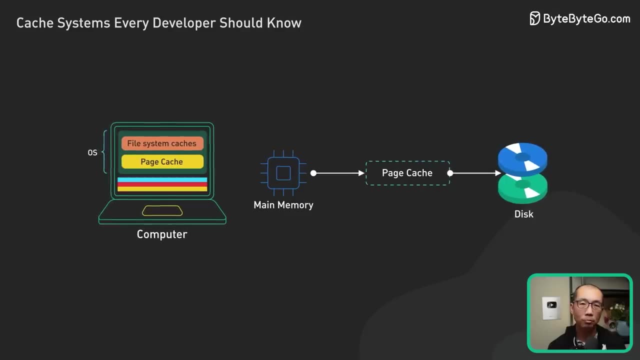 other file system caches. Page cache is managed by the operating system and resides in main memory. It is used to store recently used disk blocks in memory. When a program requests data from the disk, the operating system can quickly retrieve the data from memory instead of reading it from disk There. 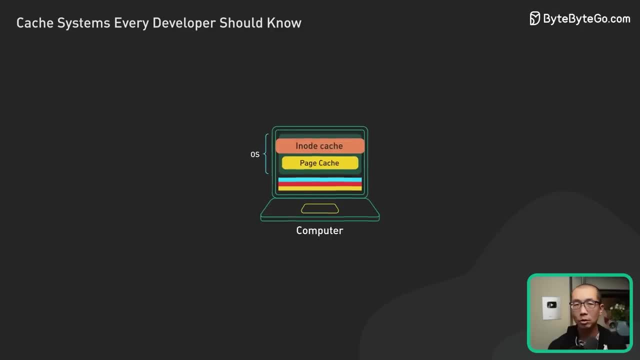 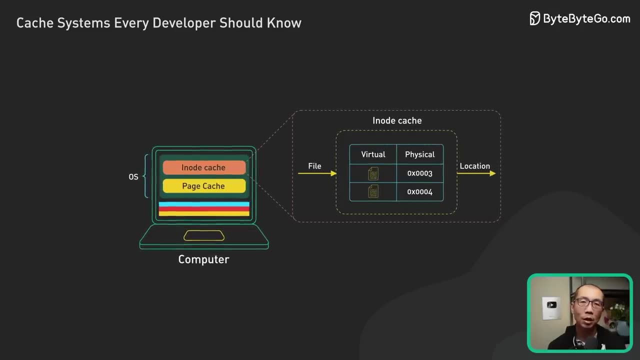 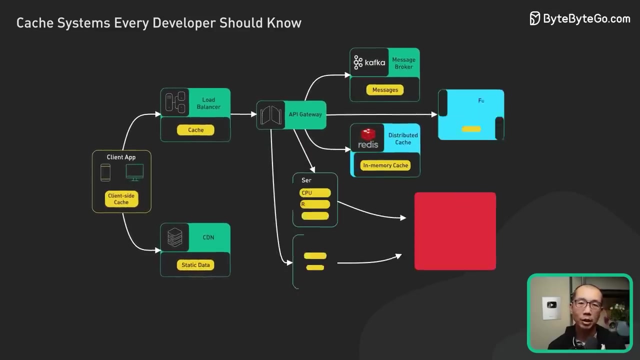 are other caches managed by the operating system, such as the inook cache. These caches are used to speed up file system operations by reducing the number of disk accesses required to access files and directories. Now let's zoom out and look at how caching is used in a typical application system. 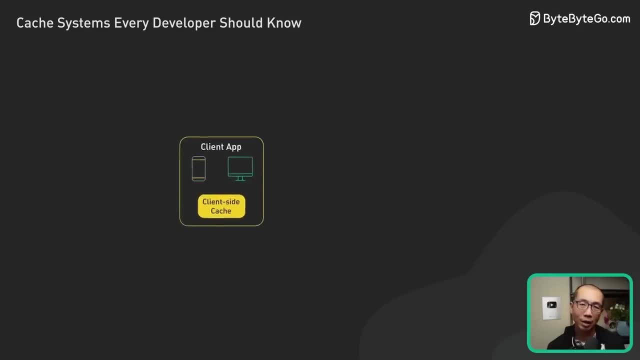 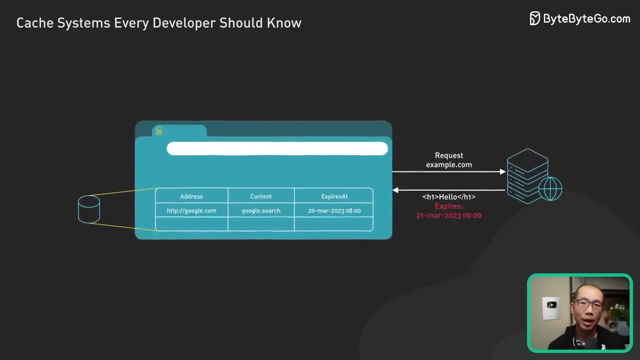 architecture On the application front end. web browsers can cache HTTP responses to enable faster retrieval of data. When we request data over HTTP for the first time and it is returned with an expiration policy in the HTTP header, we request the same data again and the browser returns the data from its cache if available. 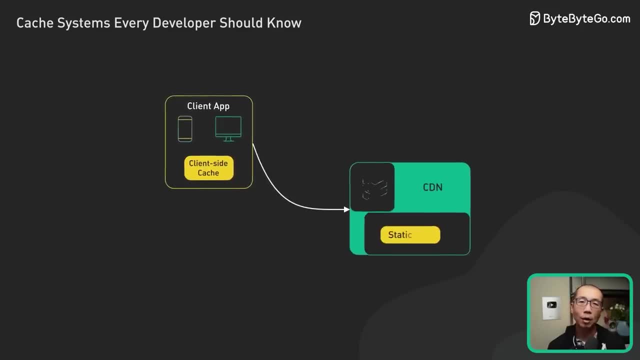 Content delivery is a very important part of the application. It is used to improve the delivery of static content such as images, videos and other web access. One of the ways that CDNs speed up content delivery is through caching. When a user requests content from a CDN, the CDN network looks for the requested. 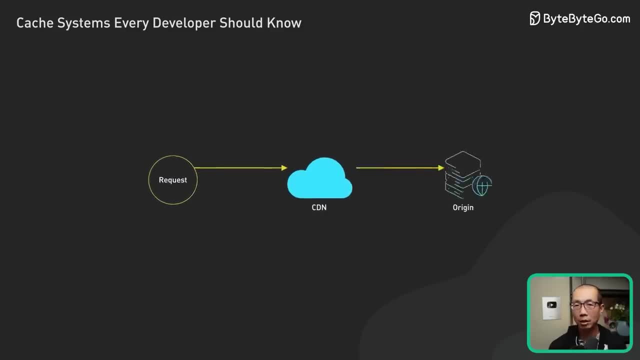 content in its cache. If the content is not already in the cache, the CDN fetches it from the origin server and caches it on its edge server. If the content is not already in the cache, the CDN fetches it from the origin server and caches it on its edge server. 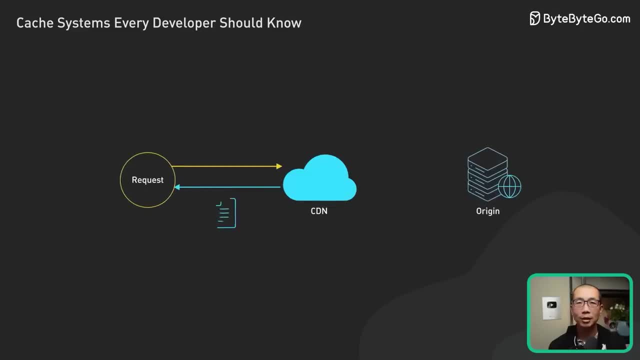 If the content is already in the cache, the CDN can then deliver its own message to the server. When another user requests the same content, the CDN can deliver the content directly from his cache, eliminating the need to fetch it from the origin server again.